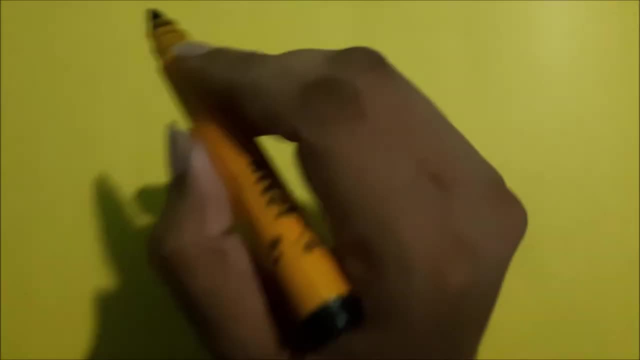 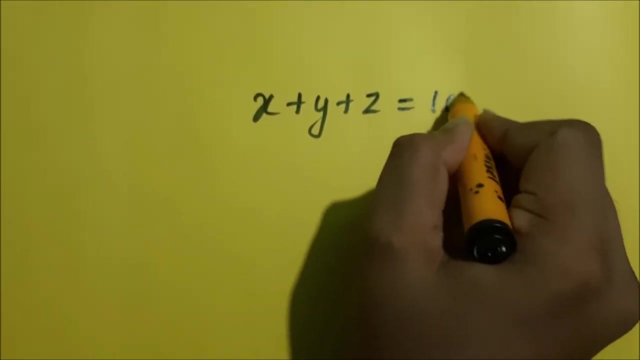 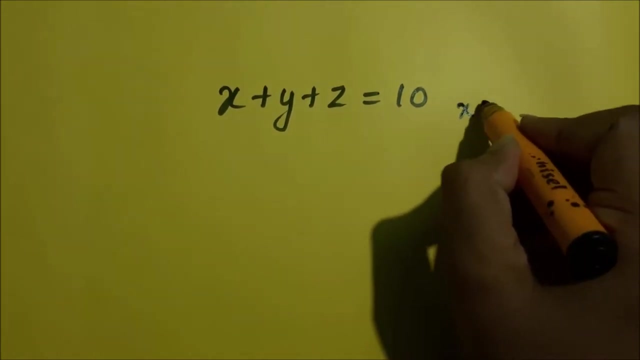 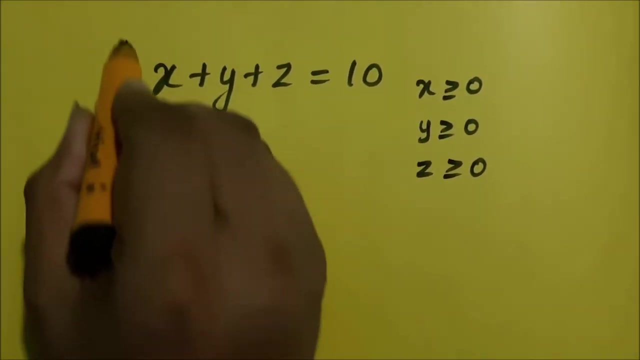 So let's start. So the question is: how many non-negative integer solutions are there for the equation x plus y plus z, equal to 10.. Alright, So the condition here is that x is at least 0, y is at least 0, z is at least 0.. Okay, And we want to find number of solutions for this equation. Okay, 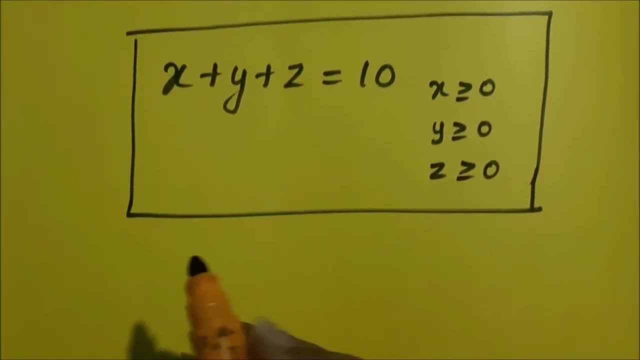 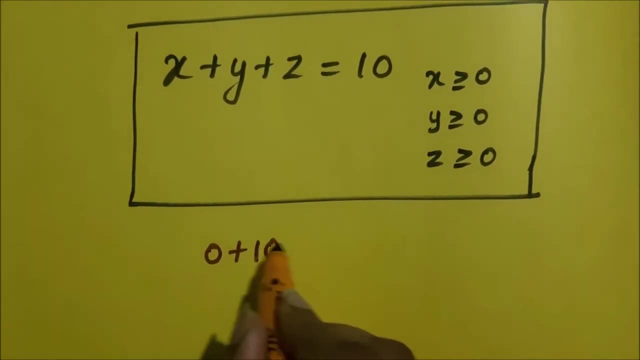 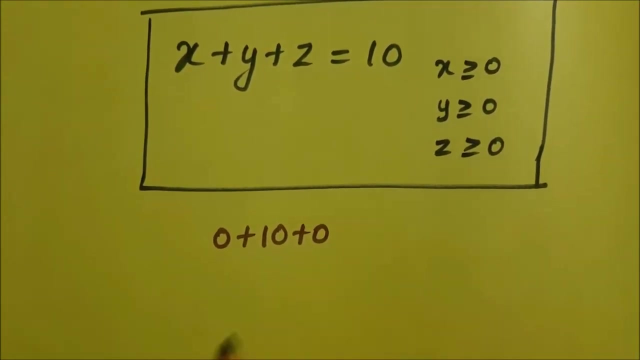 Alright, So let's show some example for the solutions of this equation. So, for example, 0 plus 10 plus 0 is a solution Right, Where x takes the value 0, y takes the value 10 and z takes the value 0. Right, So these are x, y and z. 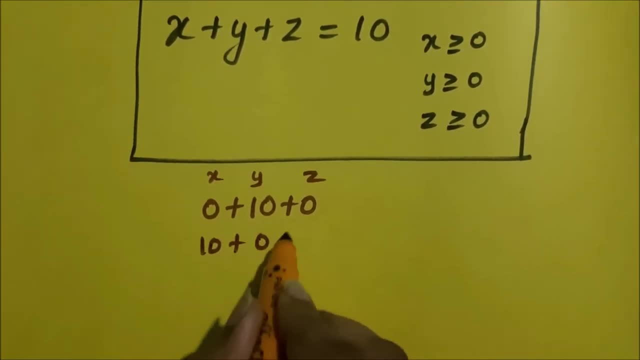 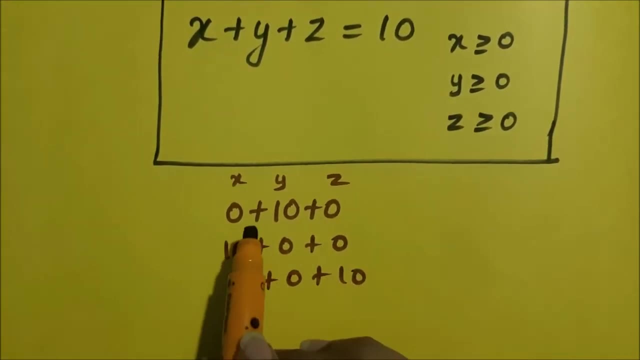 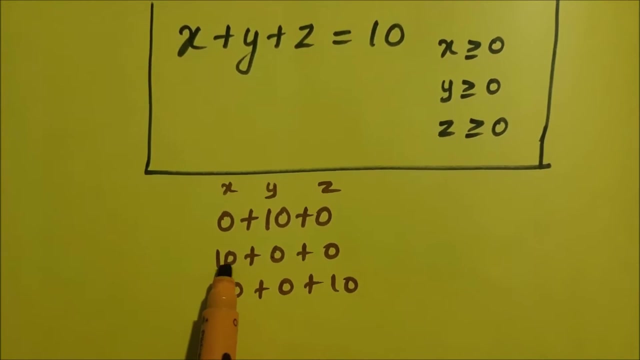 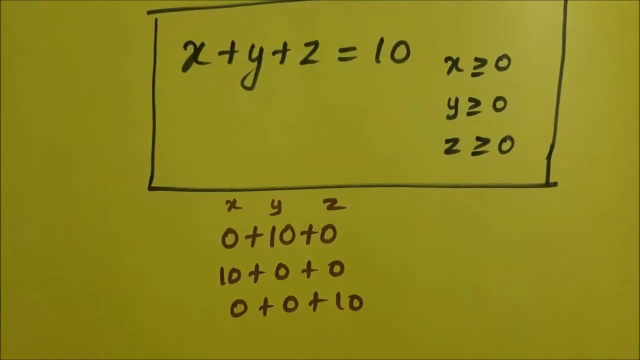 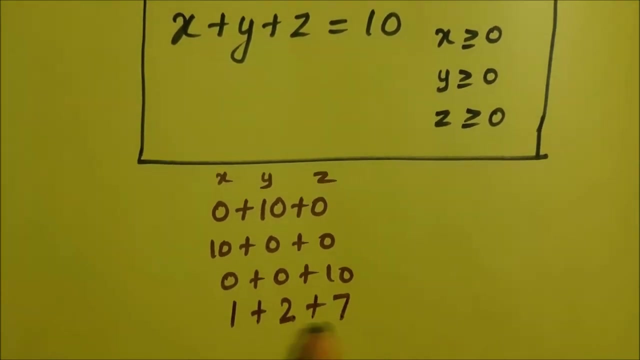 So this is different from 10 plus 0 plus 0 and this is different from 0 plus 0 plus 10.. Right, So these, even though it contains two 0s and one 10, but these three are different because it is x taking the value 10 here in this equation, It is y taking the value 10 here in this equation and it is z taking the value 10 here in this equation. Alright So. and another example is include 1 plus 2 plus 7.. Right, And this is different from 7 plus 2 plus 1, or 2 plus 1 plus 7, or whatever. Okay, 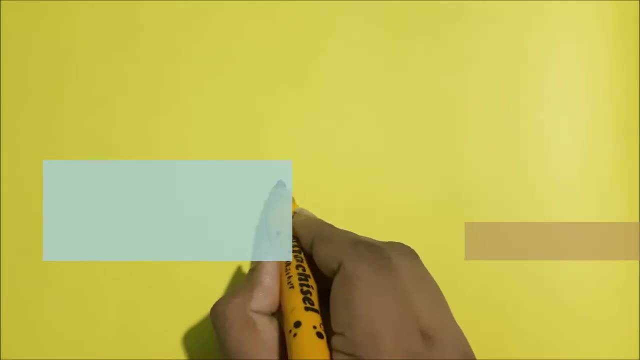 Okay. So these are some examples of the equation. So let me draw two bars. Okay, Two bars, or two dividers, whatever. So these two bars divide into three regions, Right, So here is one region, here is another region and here is a third region. Let me say, this region belong to x, this region belong to y and this region belong to z. Alright, Now what I will do is I will just draw. 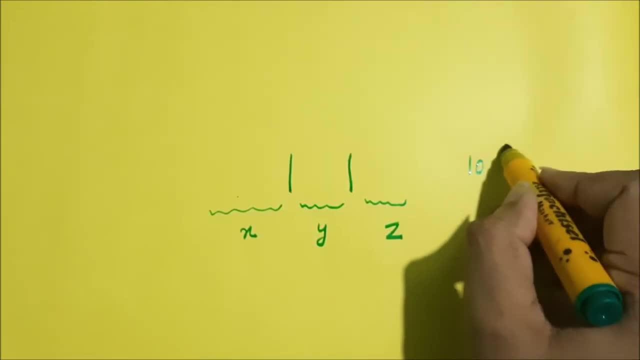 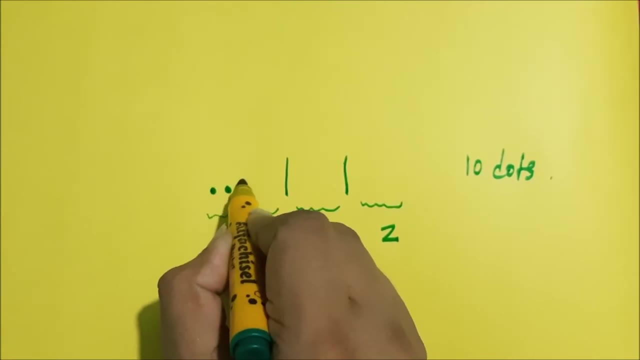 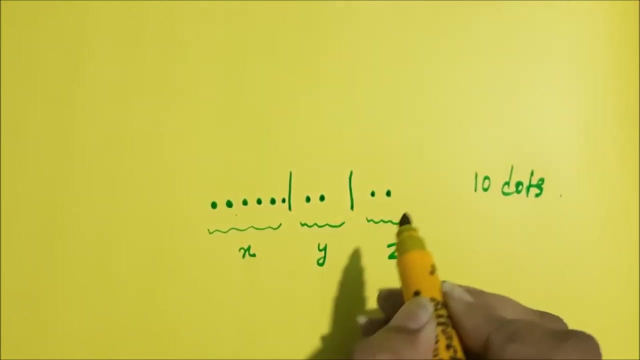 some 10 dots here. Okay, I will just draw 10 dots here. Let me do that. So 1, 2, 3, 4, 5, 6, 1, 2, 1, 2.. So here we have 10 dots Right And two bars Right Now. here this corresponds to a solution for the equation. 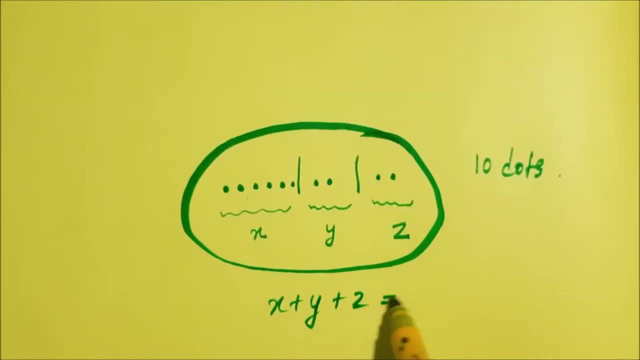 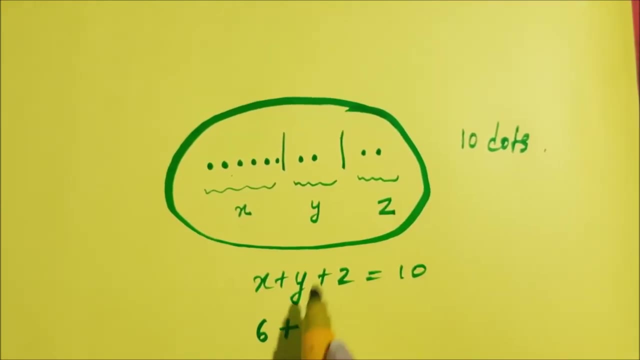 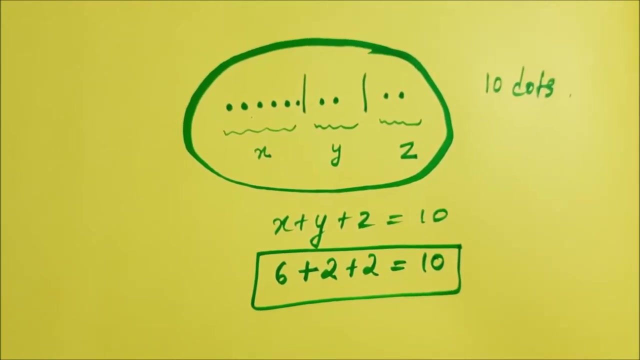 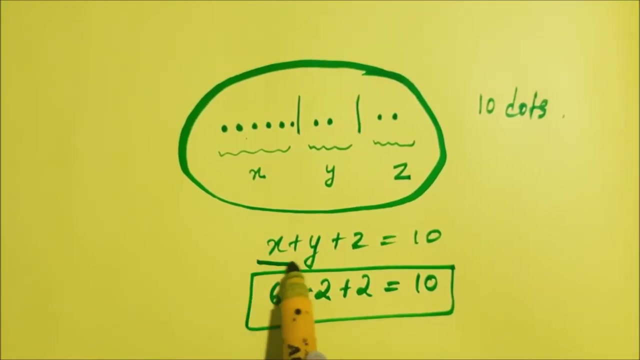 x plus y plus z equal to 10.. Where here, x takes the value 1,, 2,, 3,, 4,, 5,, 6.. Right, So 6 is the value for x and 2 is the value for y and 2 is the value for z. Right, So now, what I am trying to say is that we can reduce this problem of finding the number of non-negative integer solutions for this equation to a problem of 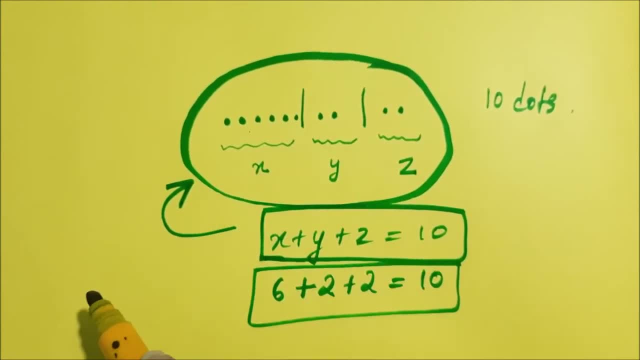 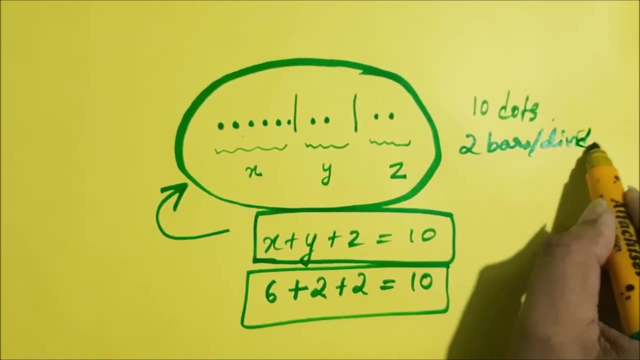 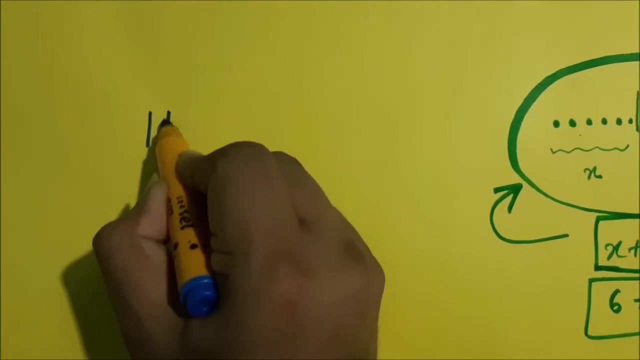 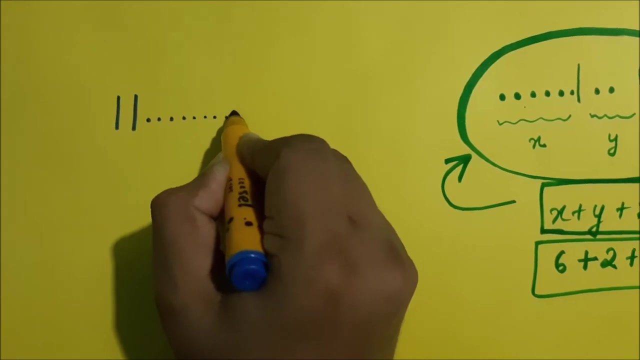 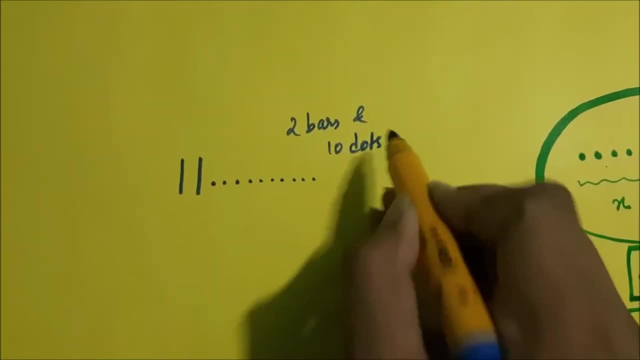 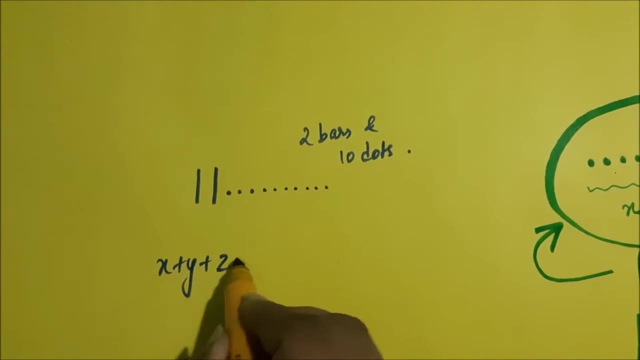 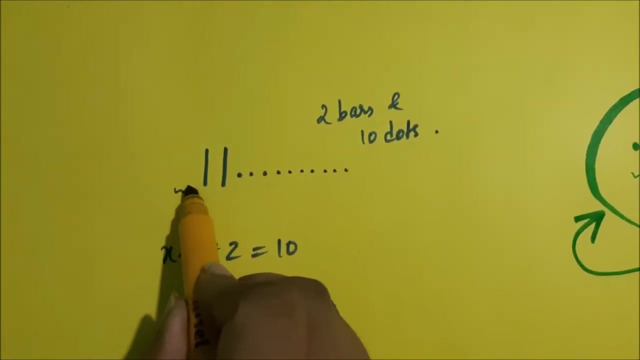 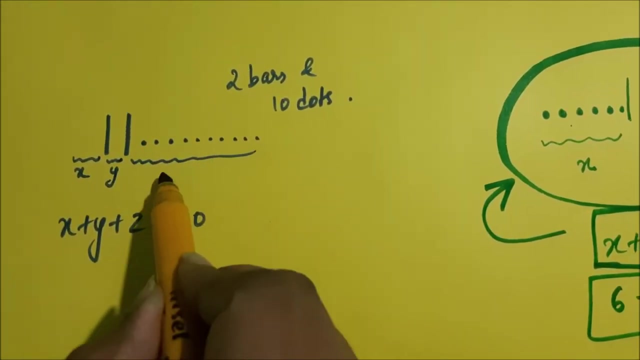 and 10 dots right. So now, what can we say about the solution for the equation x plus y plus z, equal to 10, from this arrangement? So we know that before this first bar it was the region for x, and between the first bar and second bar it was a region for y, and after the second bar we have 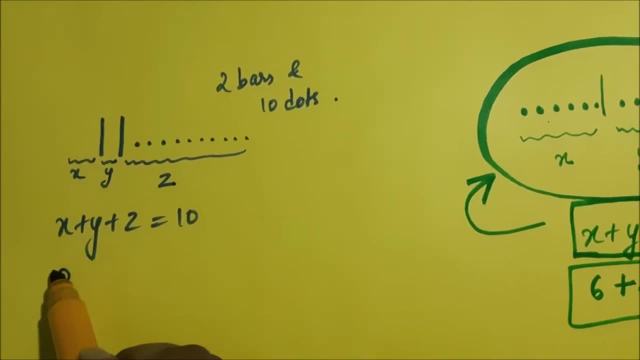 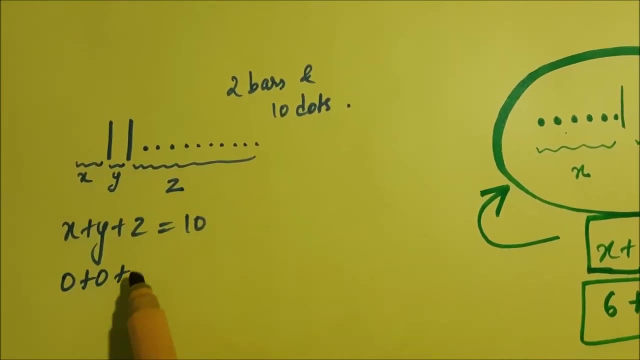 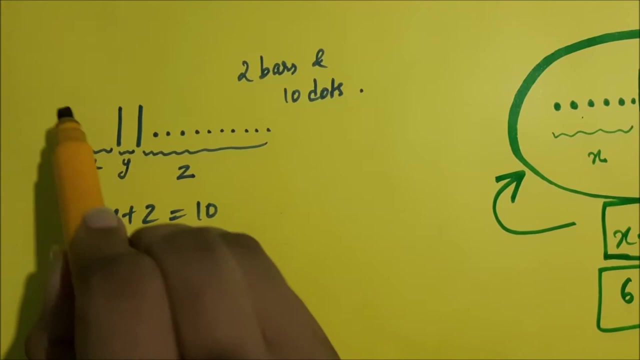 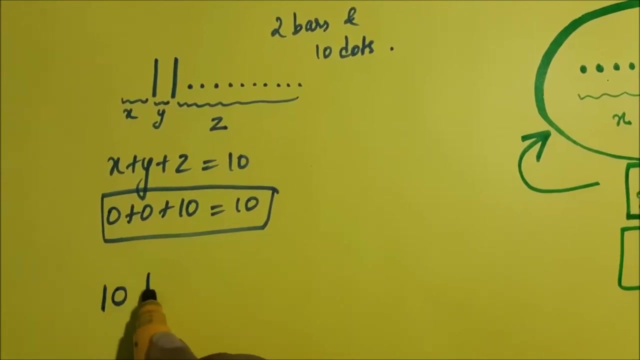 the region for z. So here x has value 0, since there are no dots in this place, and y has value 0, since there are no dots between them. these bars and z have value 10, right? So this is the solution corresponding to this arrangement, right? So what I am trying to say is that you have 10 dots and 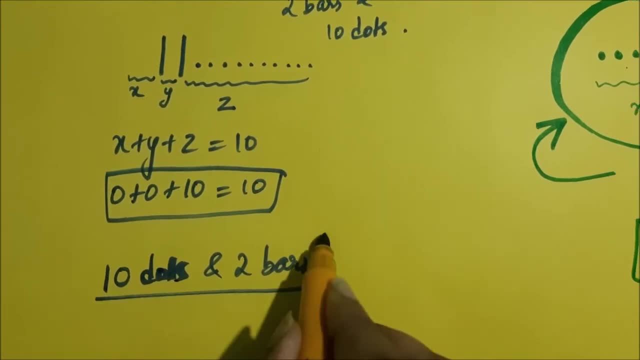 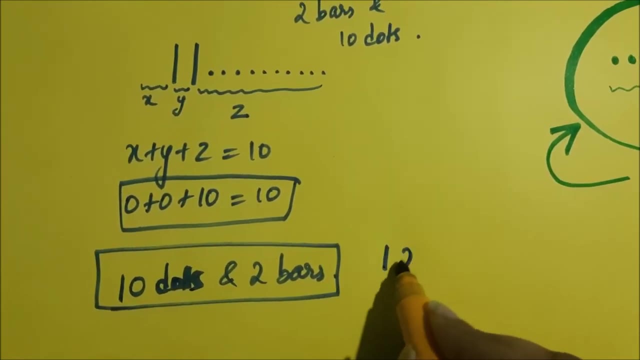 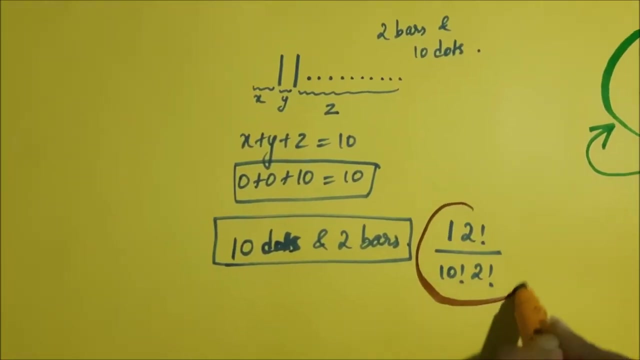 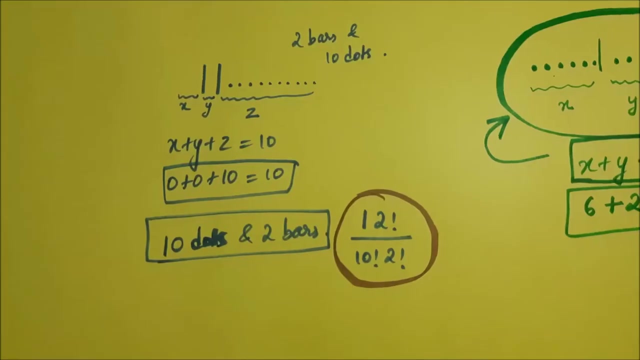 two bars, right. How many ways Can you arrange this? We know that number of ways of arranging this is nothing but 12 factorial by 10 factorial into 2 factorial. So this much number of solutions, our equation x plus y plus z, equal to 10, will have. So each of the arrangements where you have 10 dots and two bars. 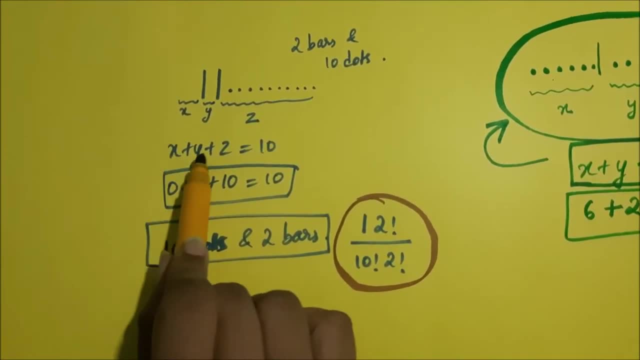 corresponds to the solution of an equation x plus y plus z. So this is the solution of an equation x plus y plus z equal to 10, where x is at least 0, y is at least 0 and z is at least 0.. 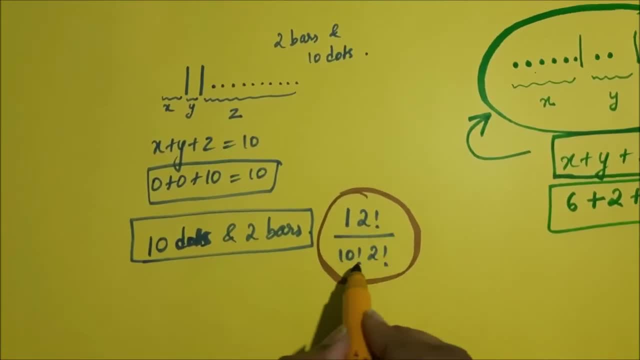 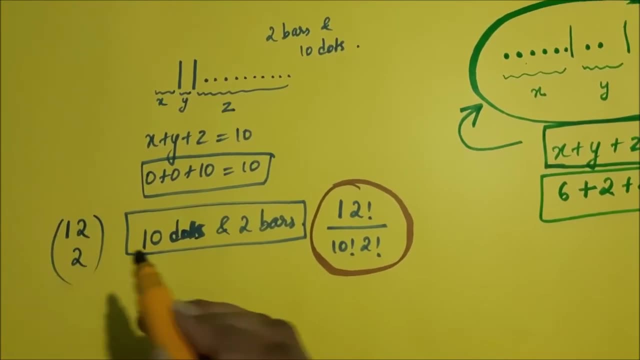 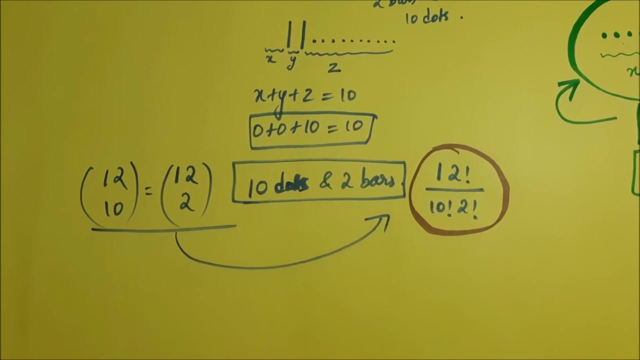 Alright Now. so what is 12? factorial by 10, factorial by 2? factorial, It's nothing but 12 choose 2 right, 12 choose 2, or we can say that 12 choose 10 right. Both are same right. So that is this number. 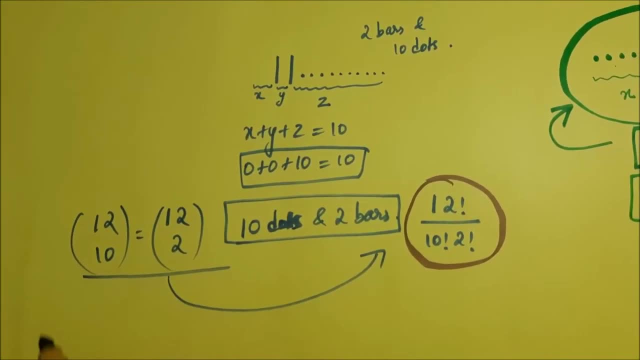 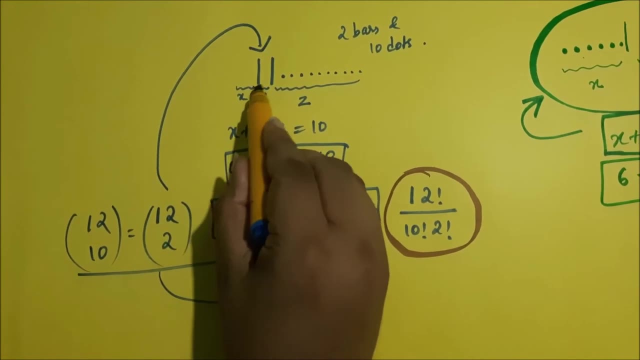 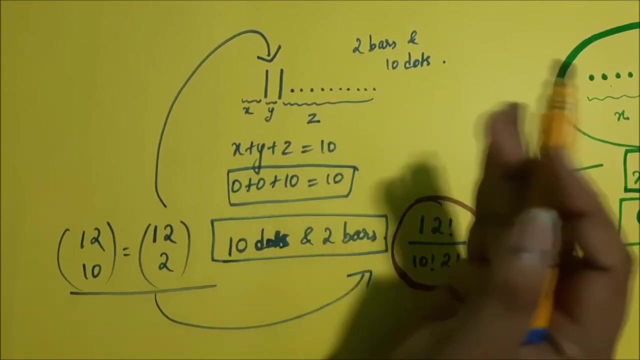 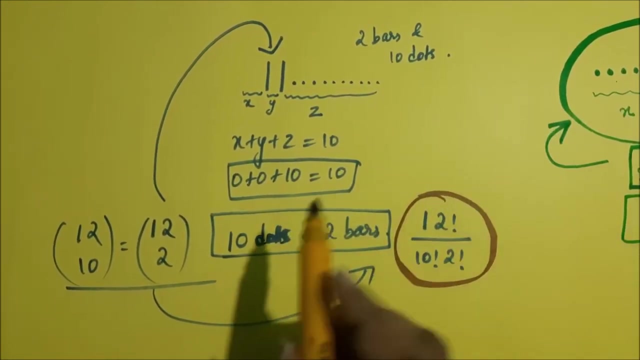 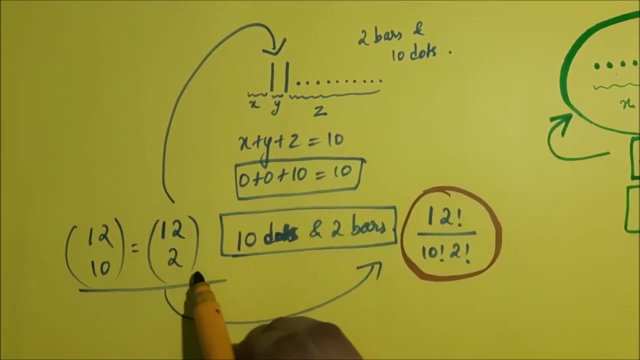 The answer is 12 choose 2, because you just need to select the placement of these two bars. If you select which place, if you select the two places where that bar can go, then that arrangement is determined right. Then we have, then we know where are the 10 dots will go right. So that's why number of ways of arranging 10 dots and two bars is also same as saying that it is 12 choose 2.. 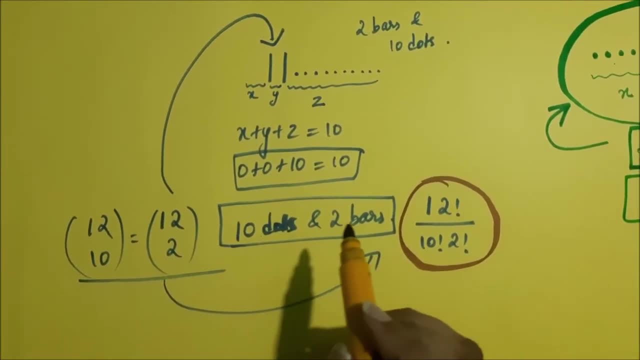 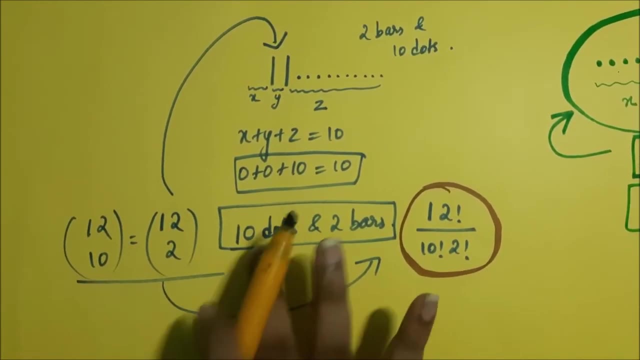 That much number of ways are there, because you just want to select the two places Where these bars can go and the remaining are will be 10 dots right. So that's why our solution is: 12 choose 2 or 12 choose 10 right. 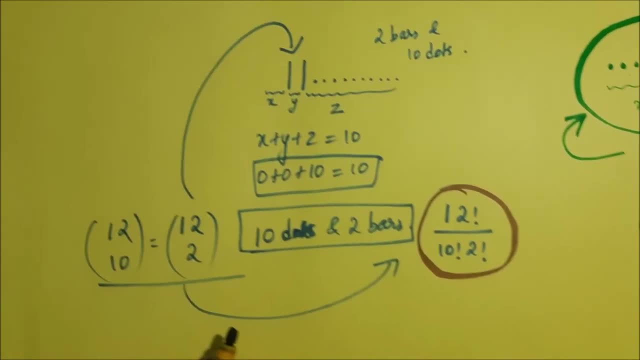 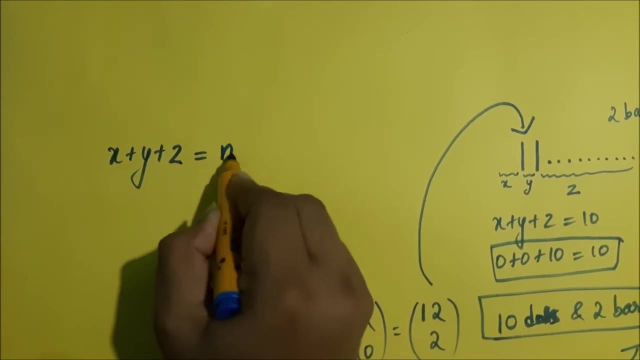 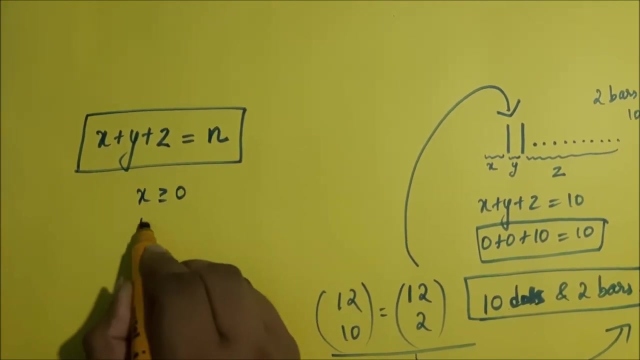 Now, in general, what can we say? Let's see. Okay, So if say x plus y plus z, equal to n. If that is the case and we want to find the number of non-negative integer solutions, That is, x is at least 0.. 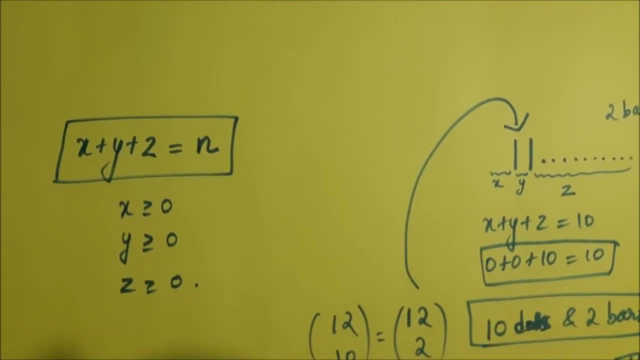 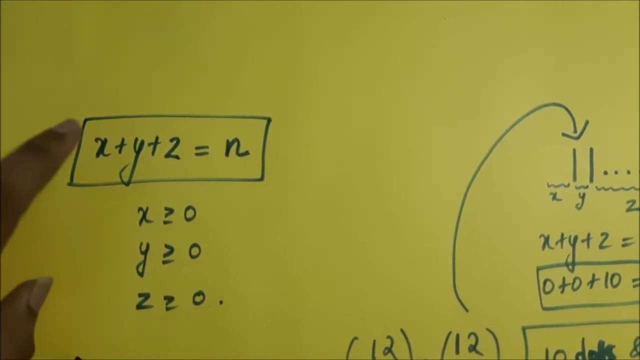 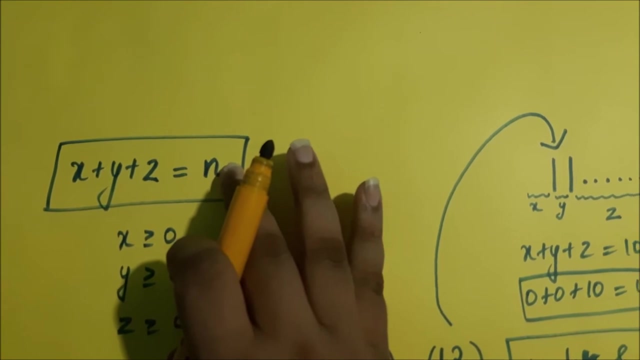 y is at least 0.. z is at least 0.. Okay, If that is the case, then what can we say? So again. so here there are three numbers, right? So depending on how many numbers we have to add up to to get this number, we decide on the number of bars. 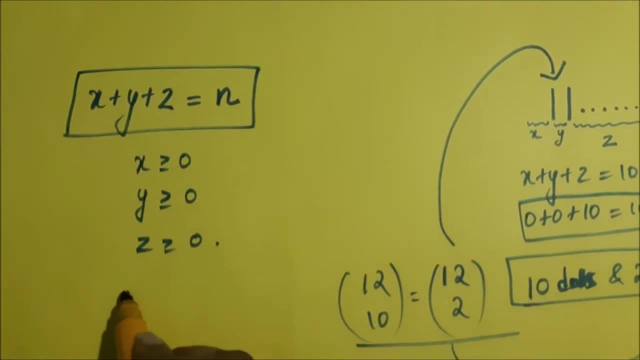 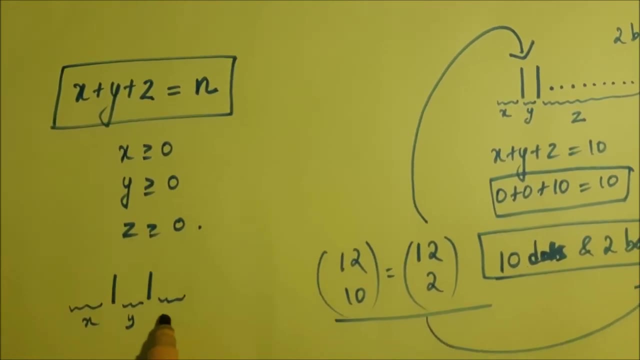 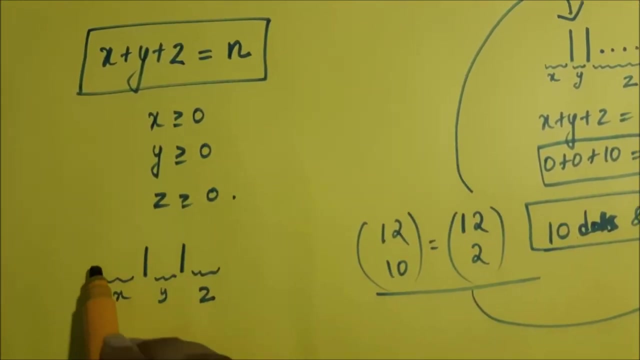 So, since there are three numbers, we can again have two bars, because we know that two bars will divide it into three regions: x, y And z. right Now we have to place how many dots. n dots we have to place. right n dots we have to place. 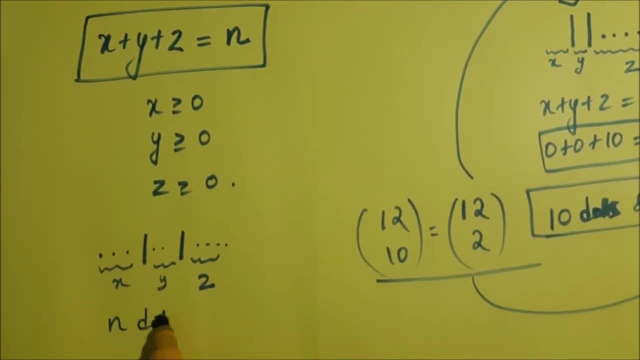 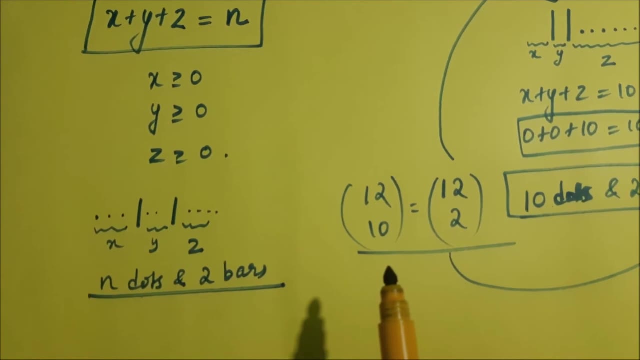 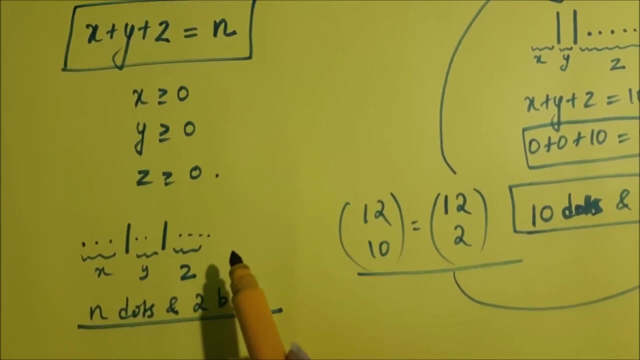 So in total there should be n dots and two bars. and how many ways can you arrange this? So that's nothing, we have to just select these two bars right and then the rest of the dots. where it will go, it's already determined, right. So the number of ways of arranging this is going to be: 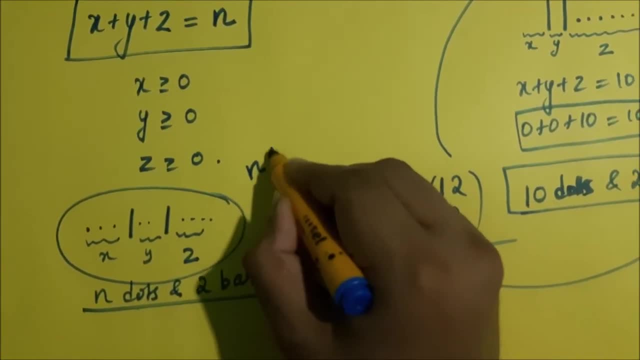 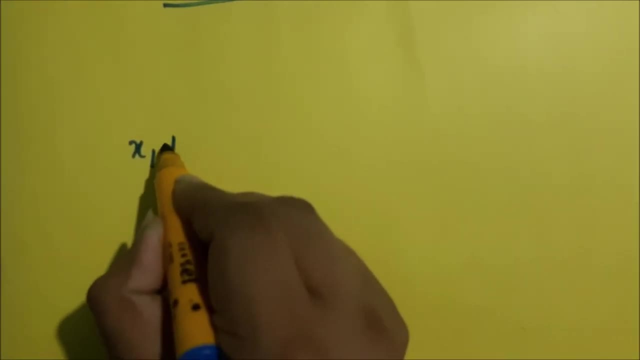 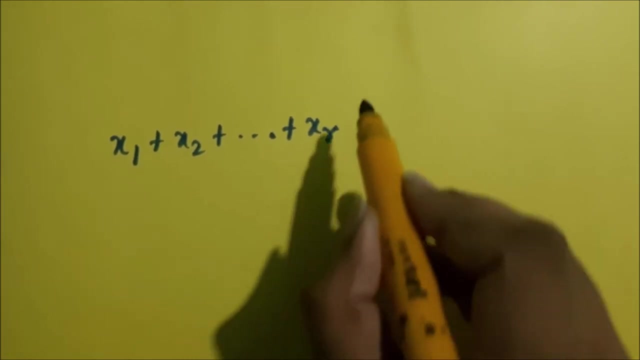 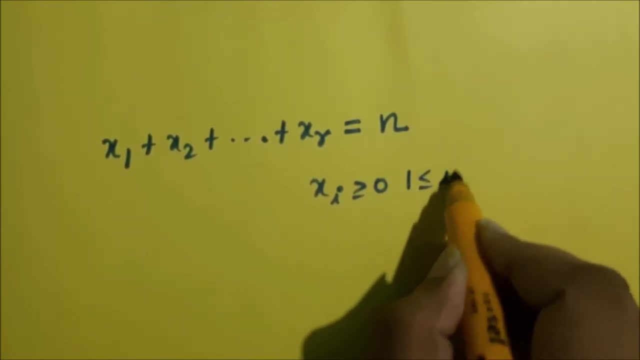 n plus 2, choose 2, right. So suppose there are x1 plus, x2 plus and so on plus xr. okay, So there are r numbers which add up to n and xi is at least 0 for 1 less than or equal to i, less than or equal to r. 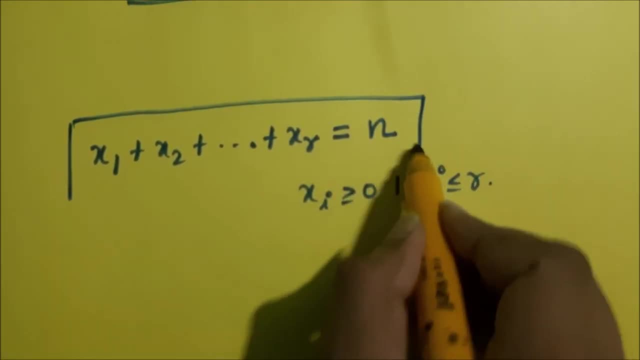 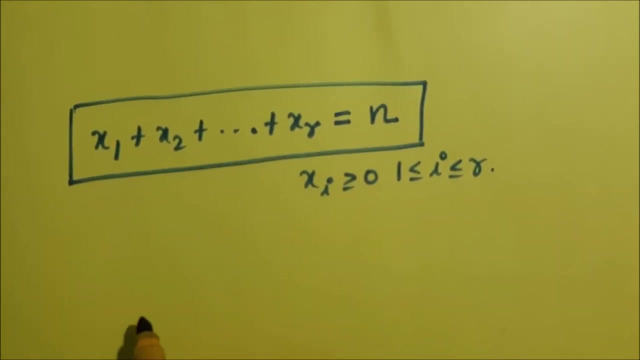 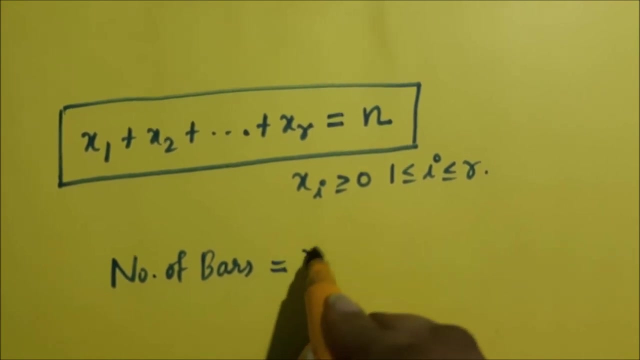 If that is the case and we want to find the number of non-negative integer solutions for this equation, Let's see. so here there are r numbers, right? So how many bars? so number of bars here will be how many it is going to be r minus 1.. 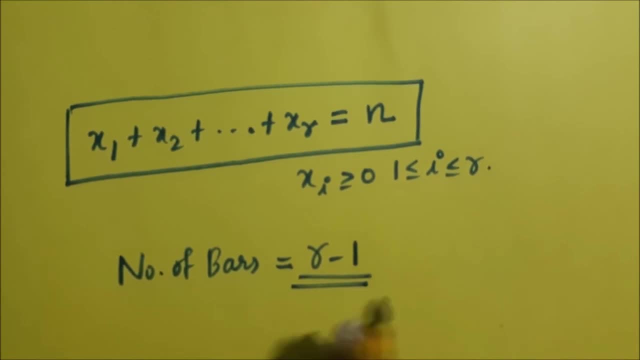 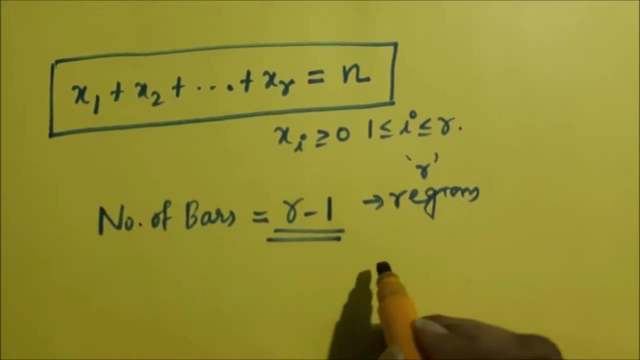 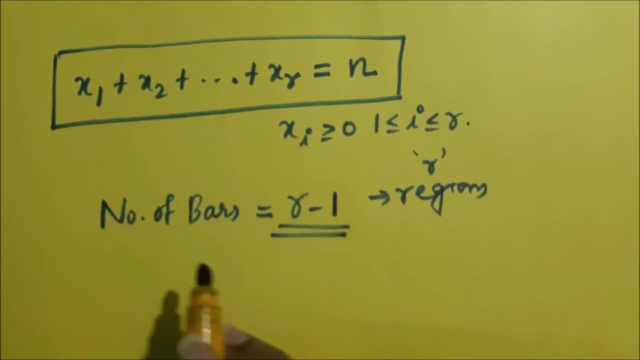 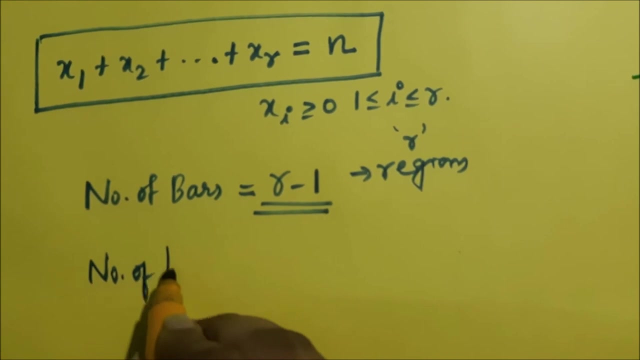 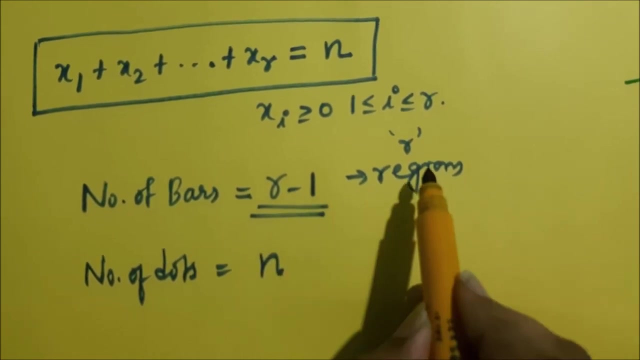 Because r minus 1 bars will divide it into r regions, right, r regions it can divide it into. okay, So that we will get the values for x1.. x2 and up to xr separately. right from that arrangement. right now we have number of bars, r minus 1 here and number of dots. it has to be n right because all the dots there should be n dots right, and r regions. so for r regions we should have r minus 1 bars and n dots, okay. 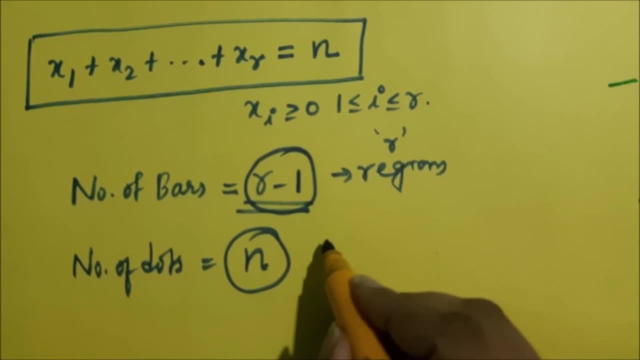 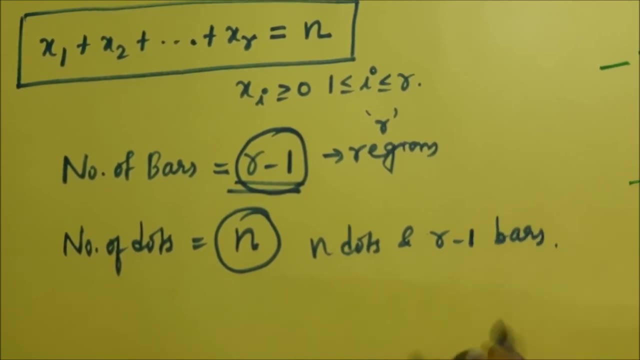 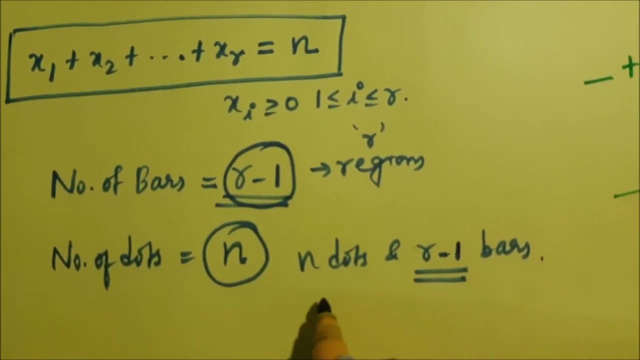 So that it should sum up to n now how many ways you can arrange n dots and r minus 1 bars. We have to just select the placements for these r minus 1 bars, right? so there are total of n plus r minus 1..